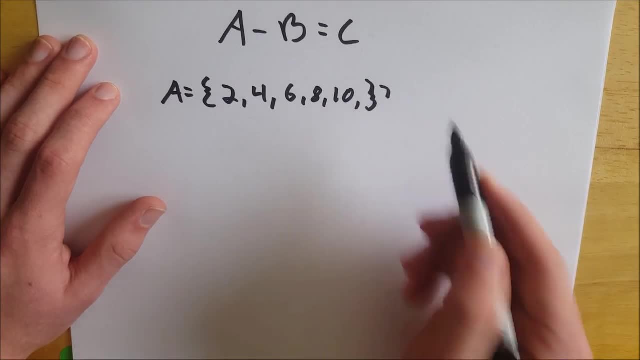 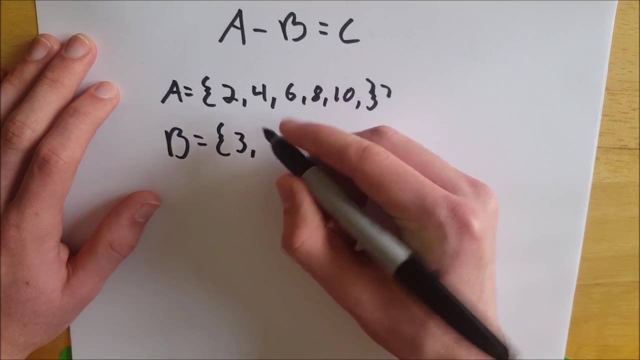 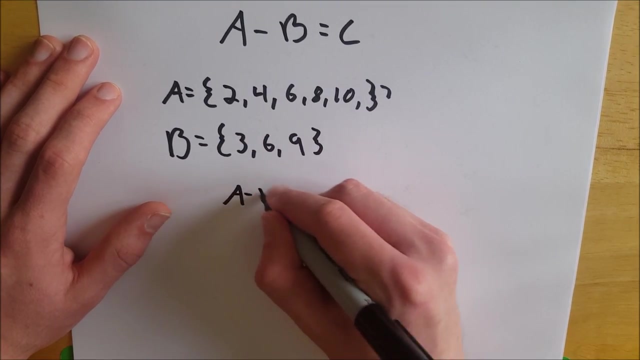 I didn't say positive the first time. I meant to Excuse that little mark I accidentally made there. Then we're going to define B as all positive multiples of 3 that are less than or equal to 10.. So we get 3,, 6, and 9.. So then, what is A minus B? 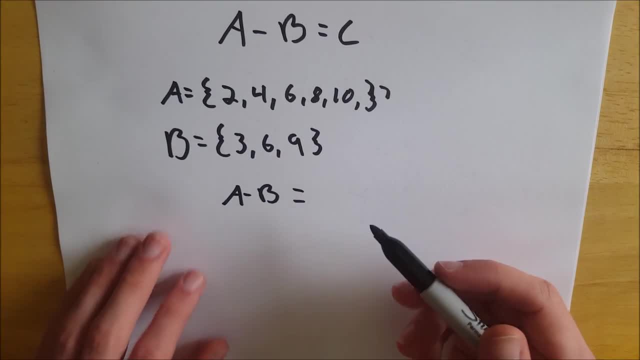 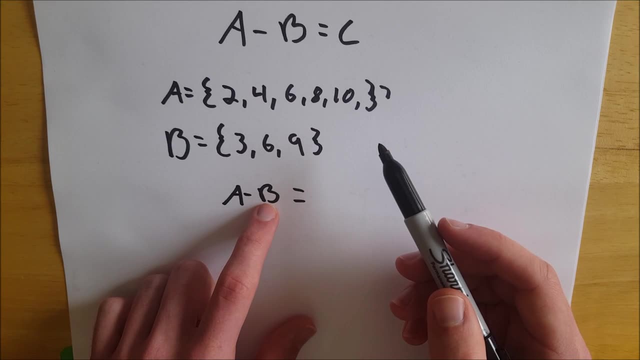 Well, when you do set subtraction, your set C is going to be all of the elements in your first set of A minus B. So we get our first set A, except missing all of the elements that it has in common with B. 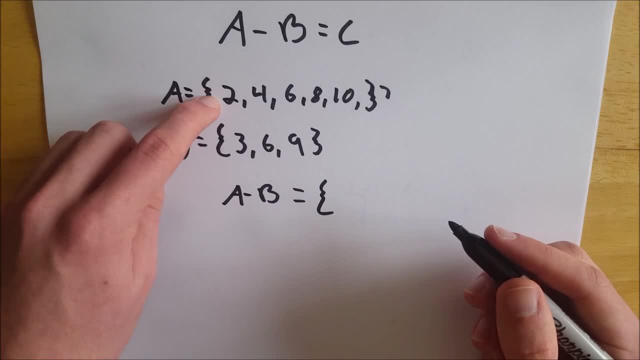 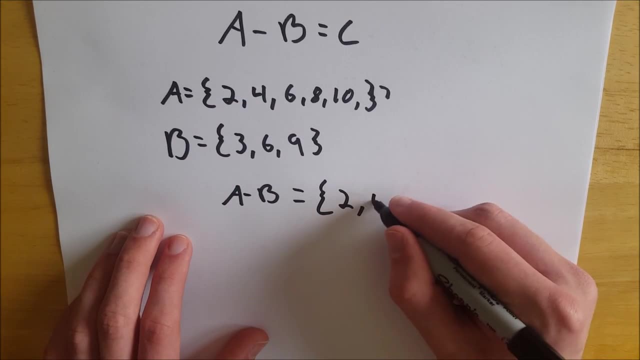 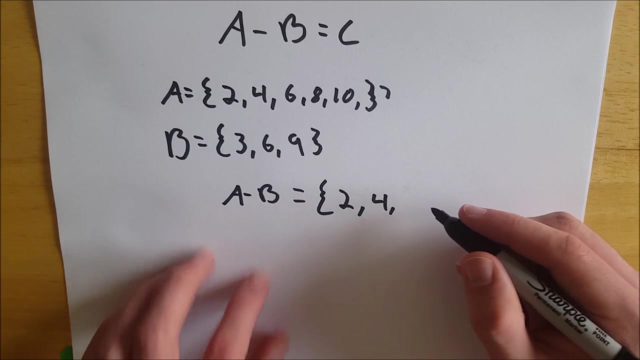 So if we go to construct this set C, we get 2, because 2 is in A and it's not in B. We get 4, because 4 is in A and not in B. We don't get 6, because 6 is in B, So 6 is subtracted, so we don't get the 6.. 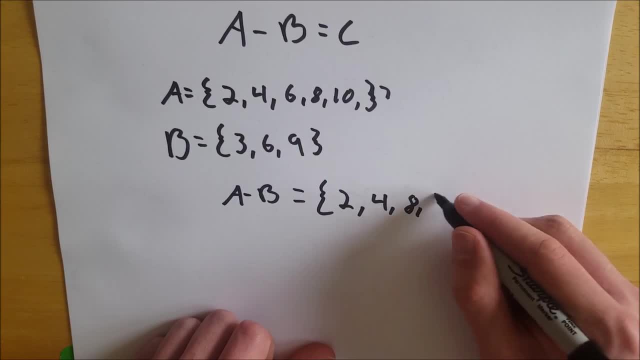 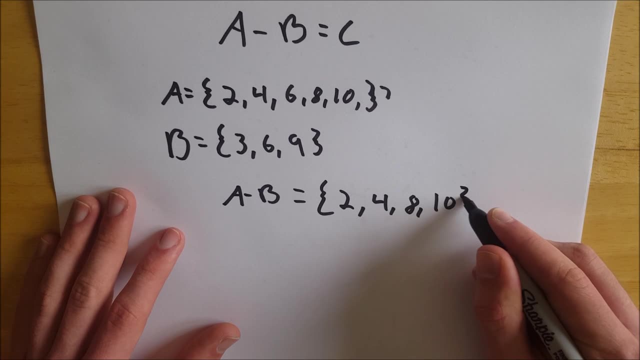 8 we get and then 10 we get. So the only one we lost was 6, because it was the only multiple of 3 that was in B that we were taking away from A. So the rule is when you're doing set subtraction. 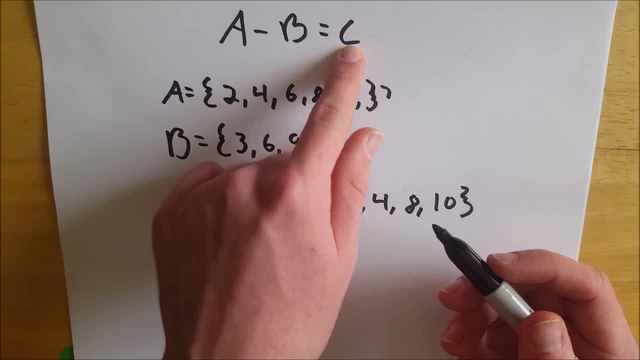 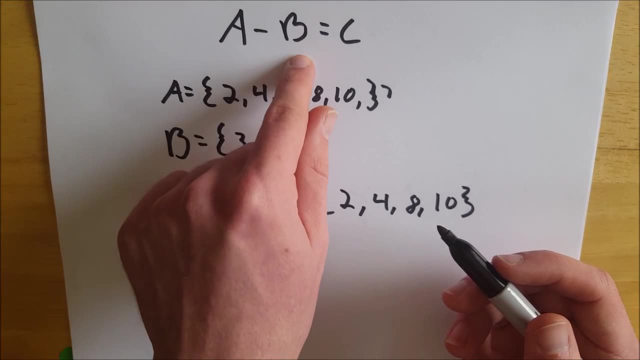 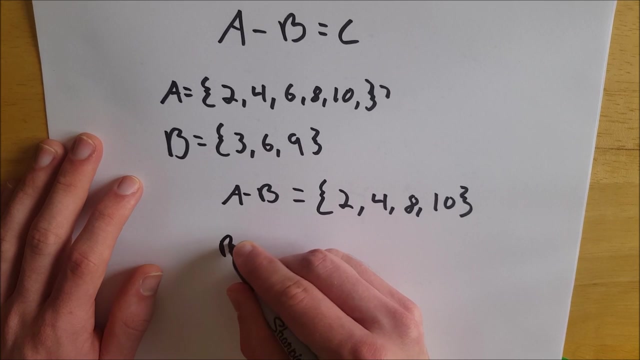 something is an element of C, the result of your subtraction, if it's an element of your first set- the set you're subtracting from- but not an element of your second set, the set you're subtracting. So let's do this in the opposite order, so you can see that as well. If we were to do B minus A, 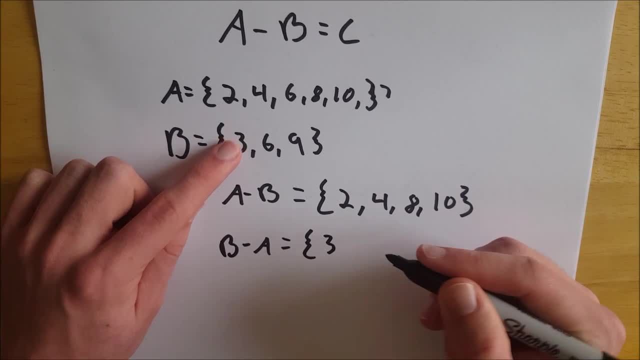 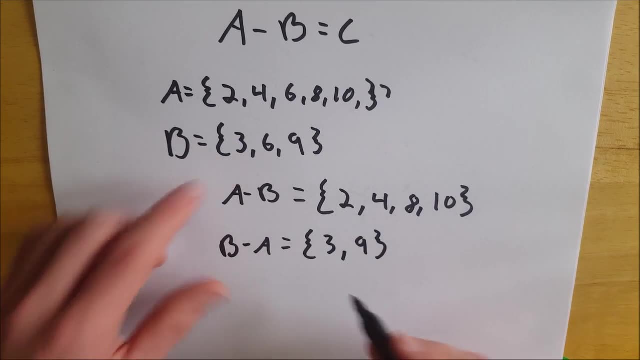 we'd get 3,, because 3 isn't in A. We wouldn't get 6,, because 6 is even so that's taken away, but we would get 9.. So B minus A would just be 3 and 9, because 3 and 9 are the only elements that 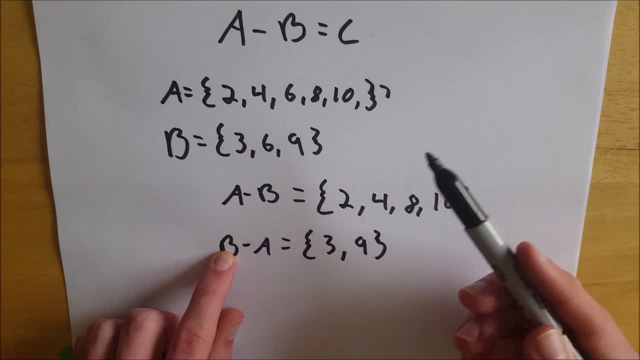 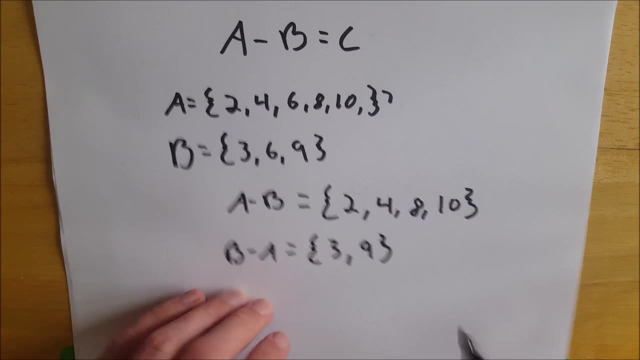 fulfill the requirements of being in B- our first set- but not in A- the set that we're taking away from B. So let me show you just a couple more weird examples so you understand how those work as well. I'll push the paper up a little bit. 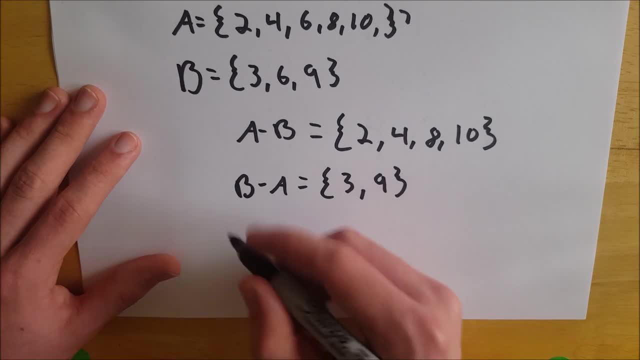 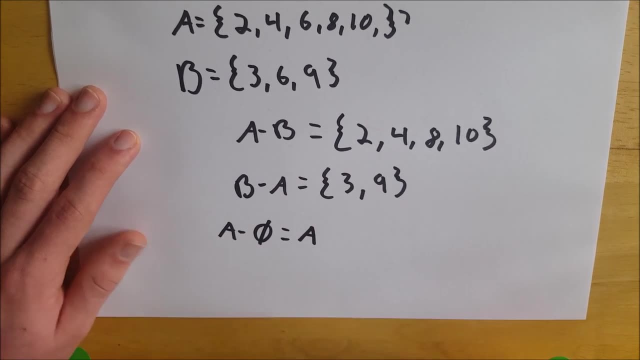 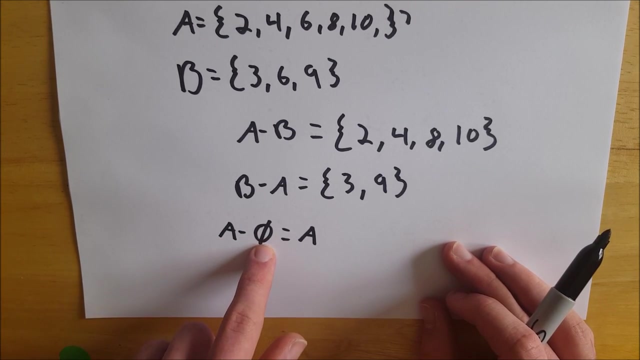 Sorry for that bloop sound. So let's say we want to do A minus the empty set. What would that be? That would just be A. The set you get from set subtraction is your original set, but missing all of the elements that are in your second set.